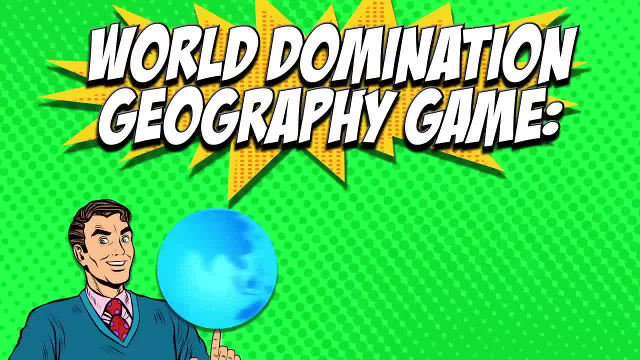 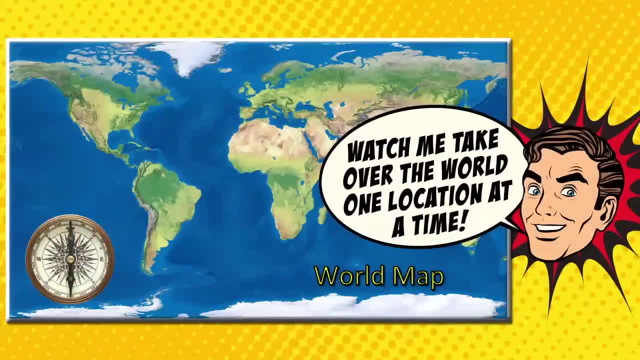 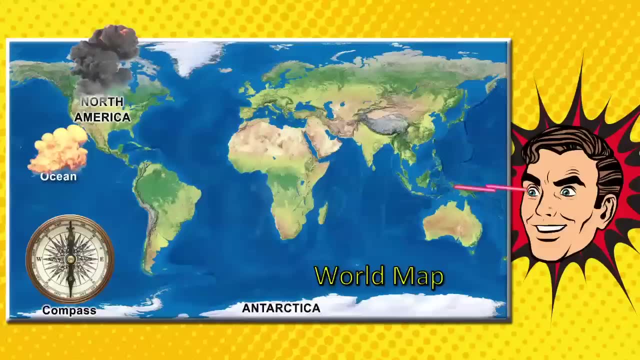 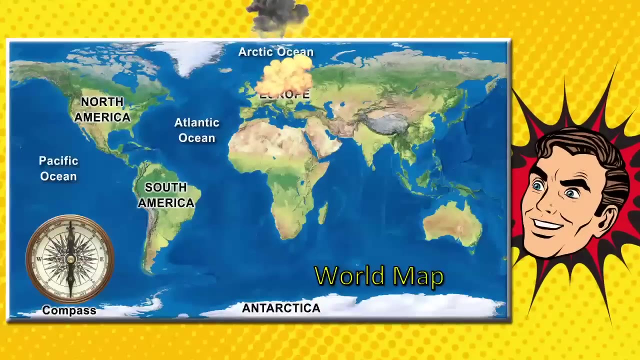 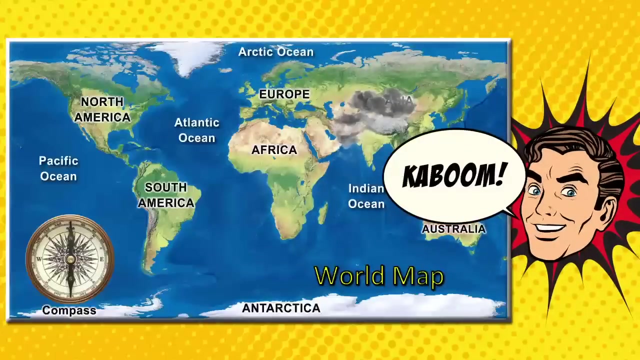 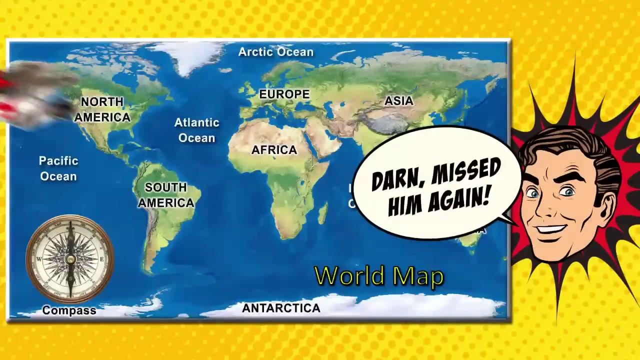 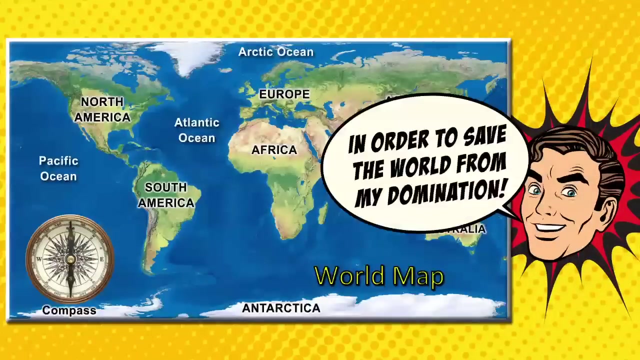 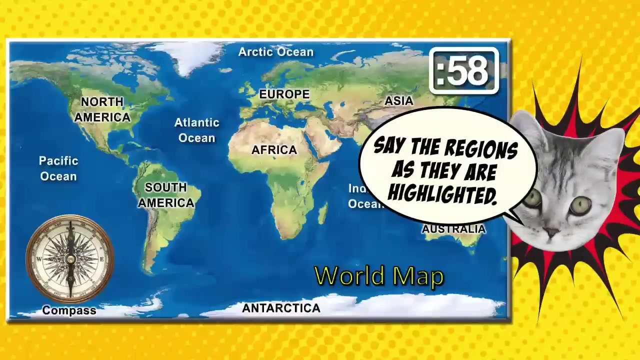 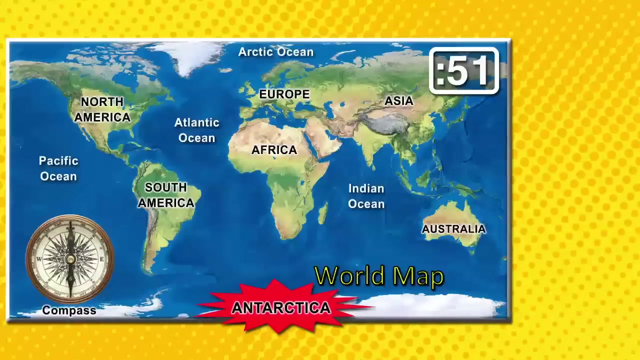 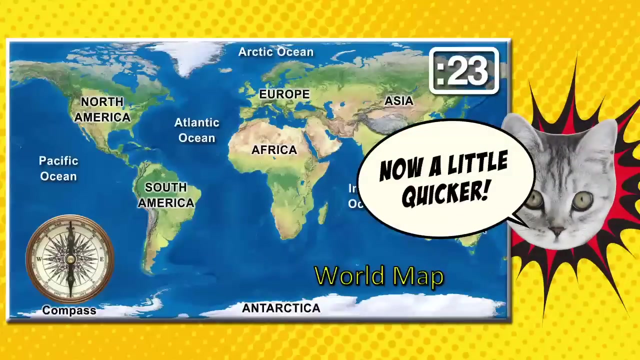 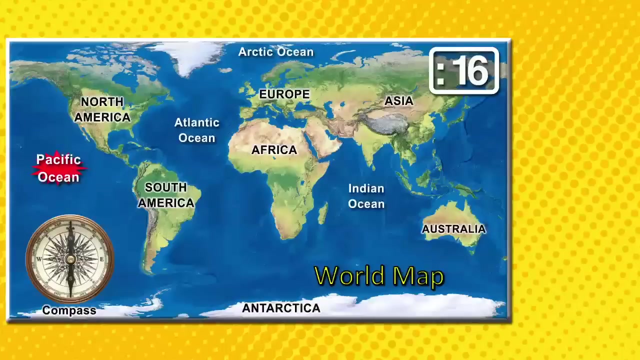 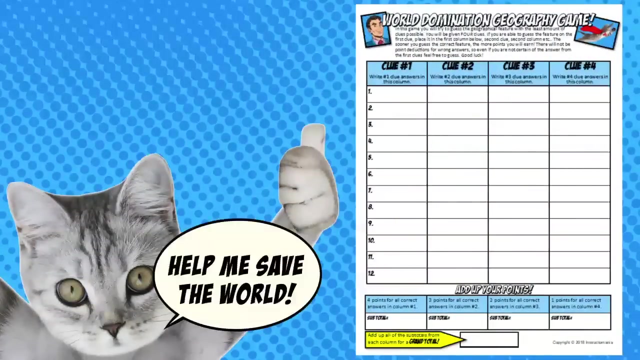 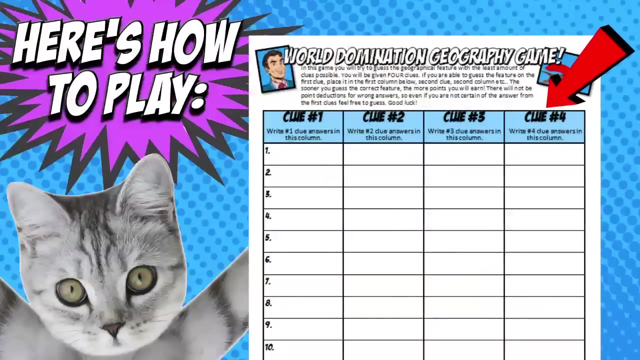 A geography game. Do you have what it takes? Will you save the world? Your correct answers may just save the world, one region at a time. Subtitles by the Amaraorg community group at Amaraorg, wwwamaraorg, wwwamaraorg. 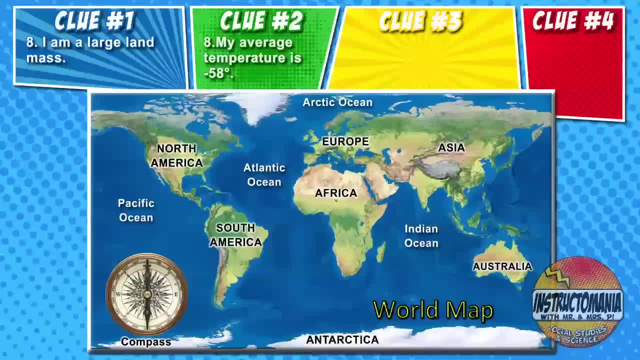 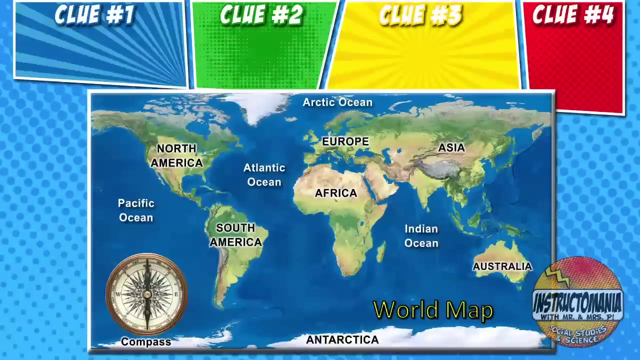 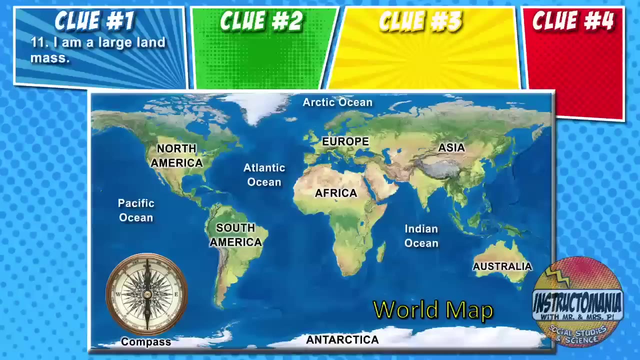